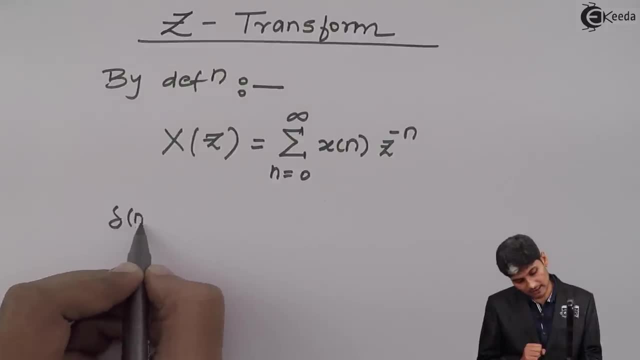 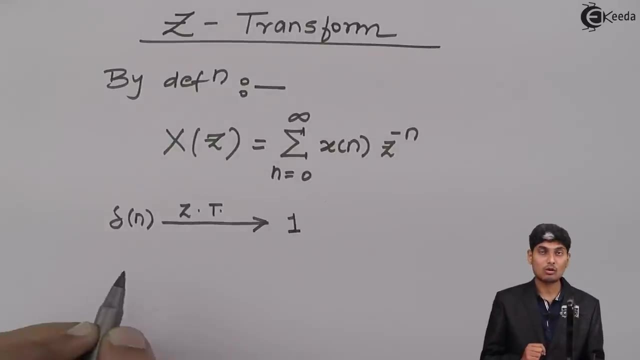 For example, if I have a signal delta n and I apply z-transform to it, then I will get the answer as 1.. If I have delta n-1,, then its z-transform is z raised to minus 1 into 1.. 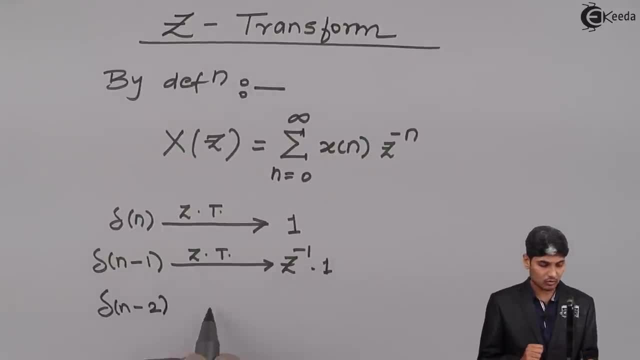 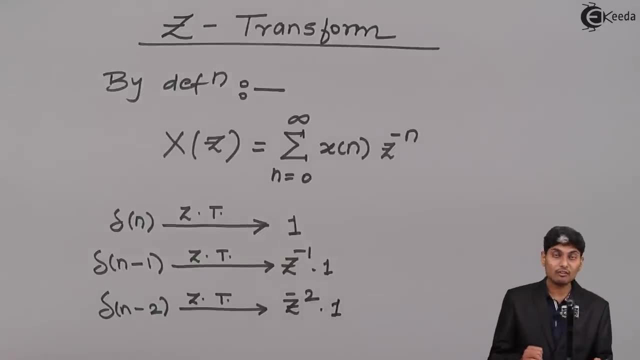 If I have delta n-2, then its z-transform is z raised to minus 2 into 1.. So if I am delaying a signal then I have to multiply by z raised to minus 2.. As we discussed earlier that minus 1 means shifting the signal to left plus shifting the signal to right. 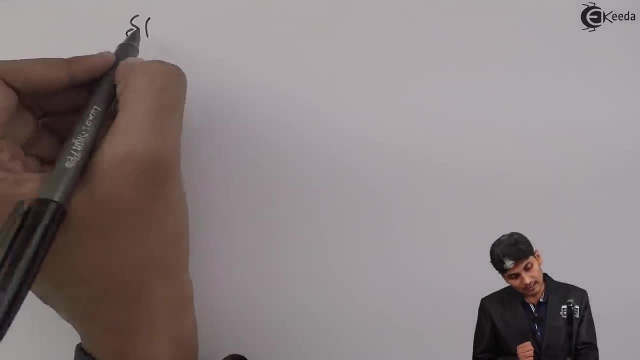 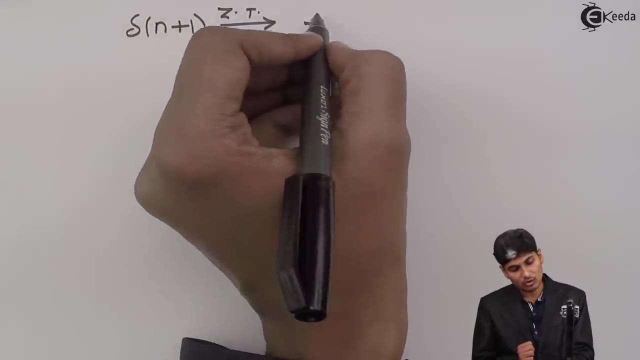 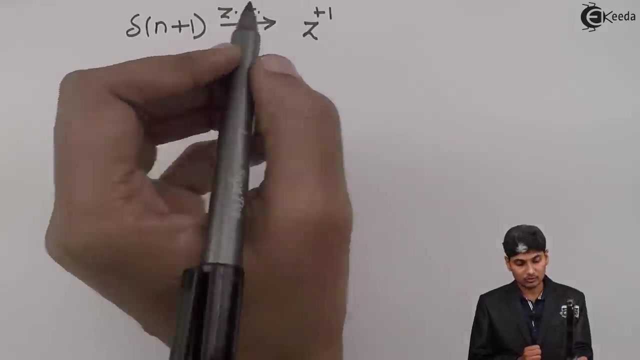 So if I have delta n plus 1, then its z-transform will be z raised to plus 1.. If it is minus over here, minus over here, It is plus over here, plus over here into 1. Delta n-1.. 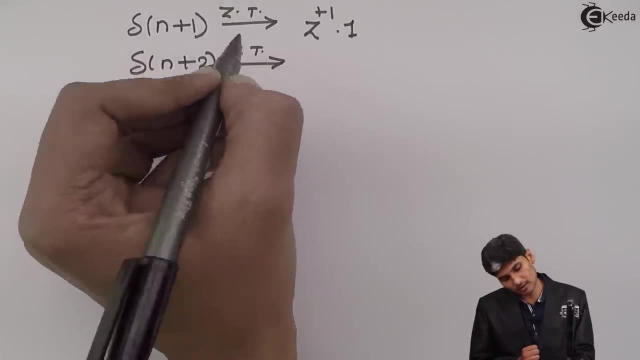 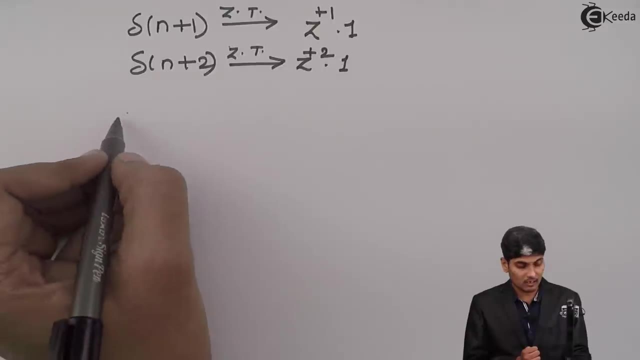 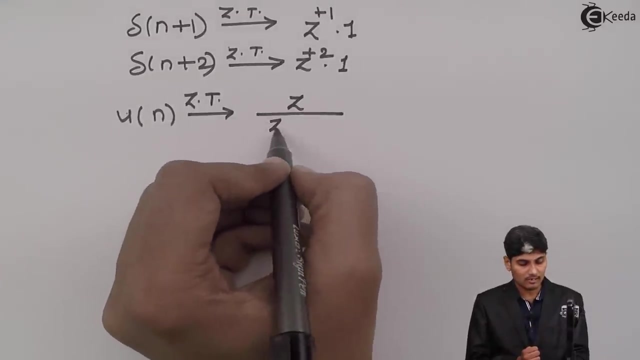 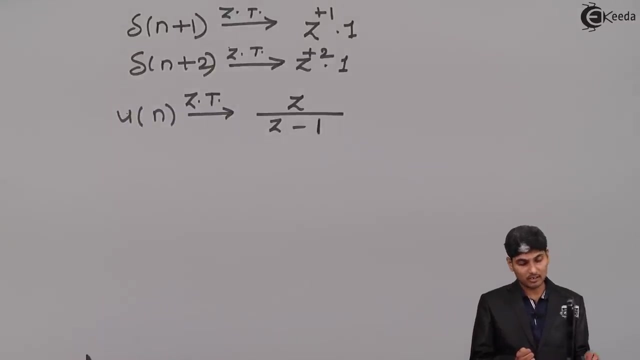 Delta n plus 2, its z-transform is z raised to plus 2 into 1.. Now let us take another signal, which is step signal. u of n. u of n z-transform is z upon z minus 1.. z upon z minus 1 is u of n. 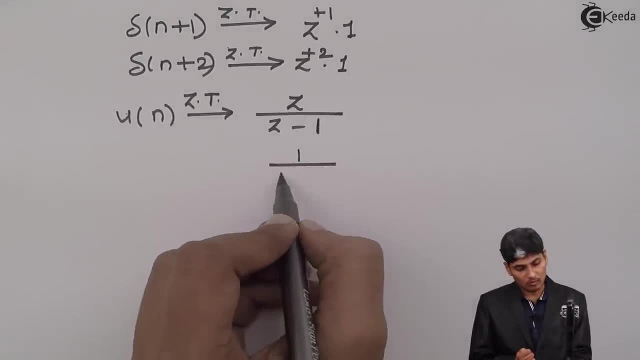 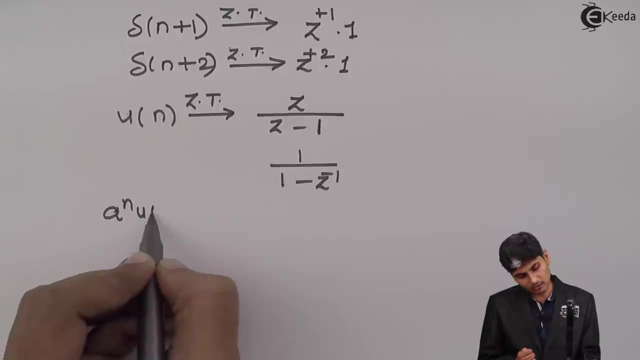 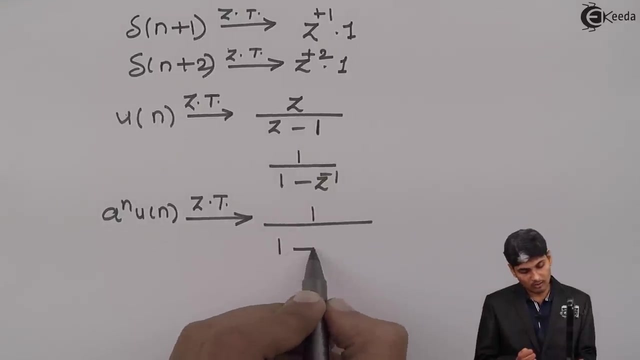 Some books write it as 1 upon 1 minus z inverse. It is one and the same. Now let us say I have a raised to n? u of n. Its z-transform is 1 upon 1 minus a z-inverse. 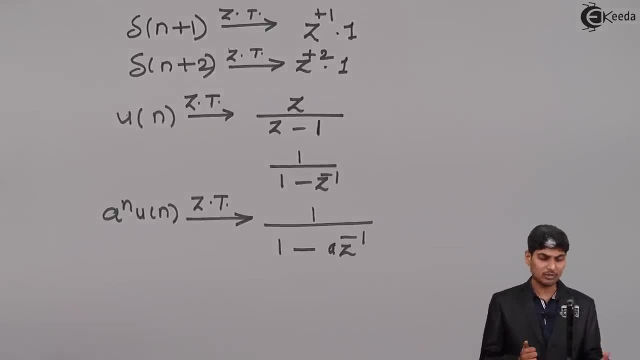 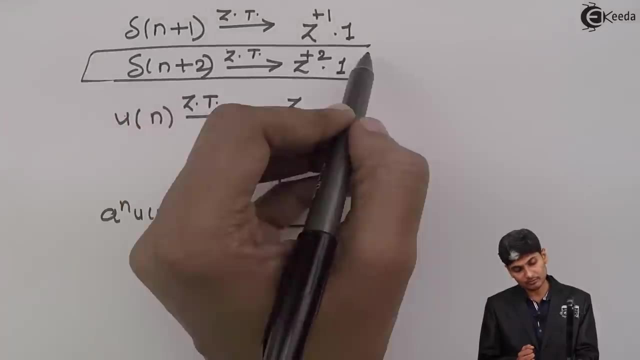 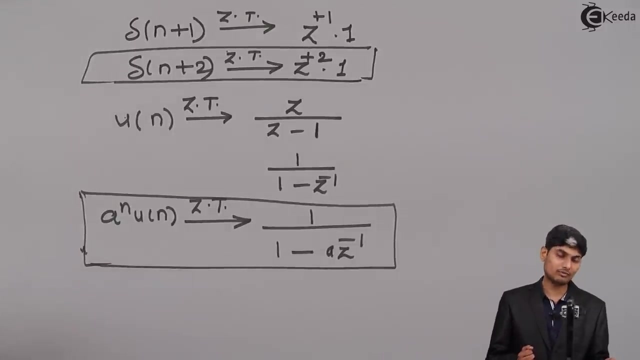 So, likewise, there is a big chart of z-transforms, but we will be using only some. That is, we will be primarily using the delaying and advancing process And a while will be always Using this formula. So these are the two basic formulas of z-transforms that we will be using very often in our systems.